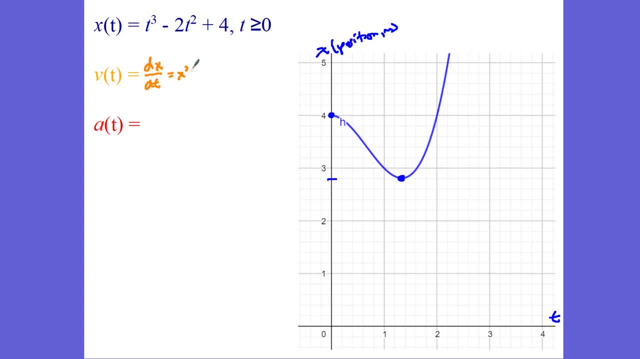 And you can see the velocity with respect to time. is the change of your position with respect to time, Or you could say your derivative of your position graph, And so let's take the derivative of this function. so we're gonna use the power rule here. We have three t squared minus 4t, and that is my new. 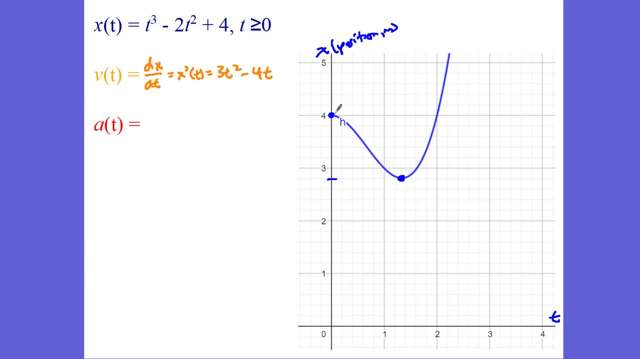 function. Um-hum, every instantaneous point in time is going to be the slope of the tangent, and so you can see how the velocity ends up getting negative, negative, negative, negative, negative, and then becomes zero, which means the velocity is zero right here, it's not moving, and then the velocity becomes positive. 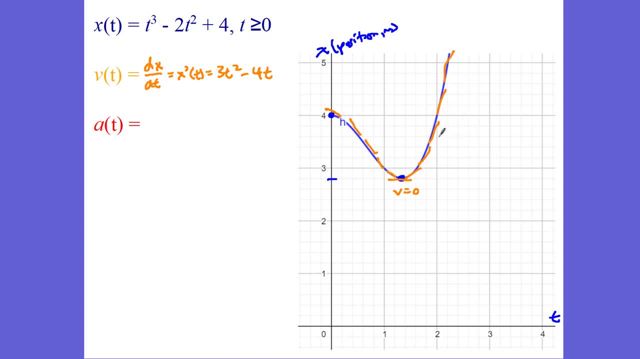 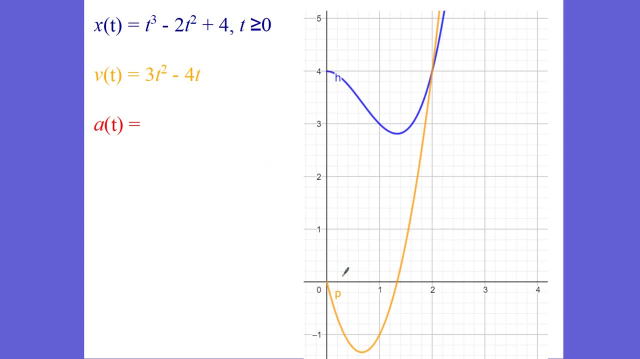 doesn't it? okay, becomes positive and so it's moving in the positive direction, and so we can graph that out. take a look at this graph. you can see how the, the, the orange is the velocity with respect to time, okay, and you can see my velocity starts at zero because my slope of my tangent is: 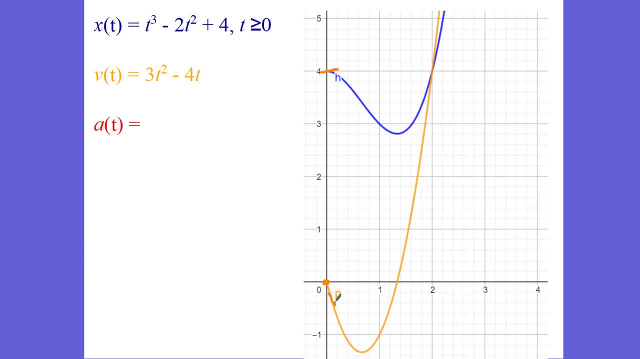 about zero here, okay, and then you can see the velocity ends up being negative. now what does negative mean? it doesn't mean it's moving slow, it means it's moving backward. and you can see, then the velocity becomes a their becomes the most negative. the steepest slope, the fastest it's going right here. and then you can see: 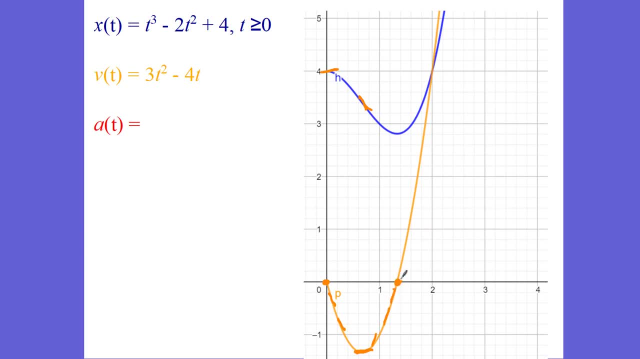 then it starts to slow down, and now, right here in my velocity graph, you can see my velocity is equal to zero right here. what does that mean? the slope of the position time graph is zero, which means it has stopped, and now it's speeding up in the positive direction and so it has changed. 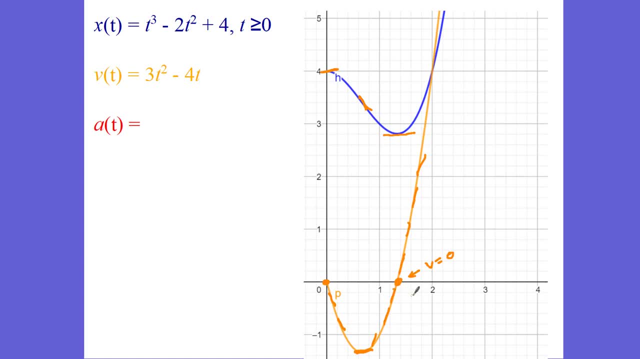 directions. so when your velocity time graph goes from negative to positive, that means you're changing direction. you're changing direction. so you can see in the velocity time graph: when your velocity is equal to negative, that means it is moving backwards, okay, and then when your velocity is positive, that means it's moving forwards, okay. 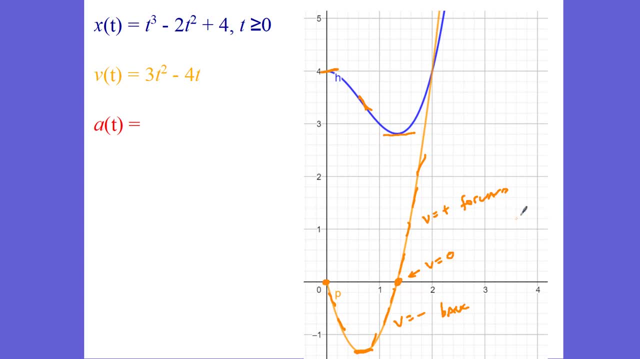 so there's four different ways that your velocity time graph works. okay, whether it's speeding up or slowing down. remember speed is a scalar quantity. velocity is a vector quantity, so velocity has direction involved. speed means you can see from zero meters per second. remember we're dealing 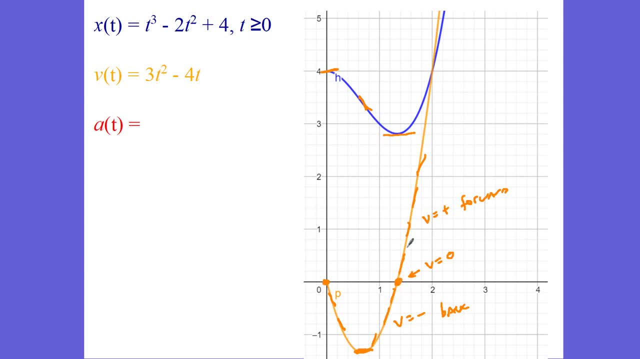 with velocity. here we're speeding up, then, right here we start to slow down. okay, then we start to speed up again after it. okay, now, remember, you can find out. the acceleration, knew. velocity with respect to time is the derivative of the position with respect to time, or x prime t. well, the acceleration with respect to time is the change of the velocity with respect. 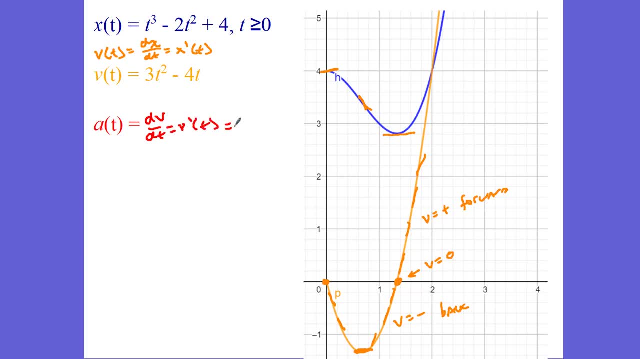 to time, or v prime t, or you could say the second derivative, the second derivative: d squared, x over dt squared, the second derivative of the position with respect to time. so let's take this velocity time graph or function and let us find the acceleration. so we got the power rule, we get 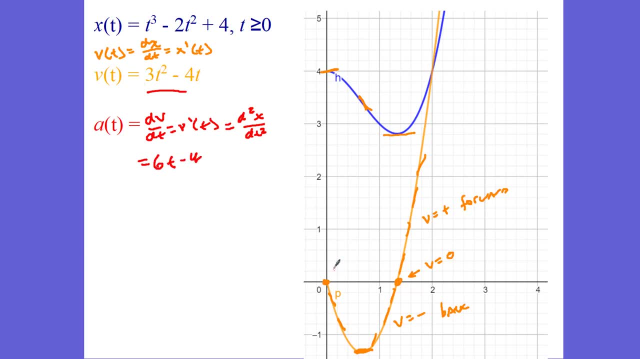 6t minus 4, and so you can see how the acceleration is a linear function here. okay, i hope you can see the x, that the position function is a cubic function, the velocity function is a quadratic function, a squared function. the acceleration is a linear function. okay, and so you can see how. 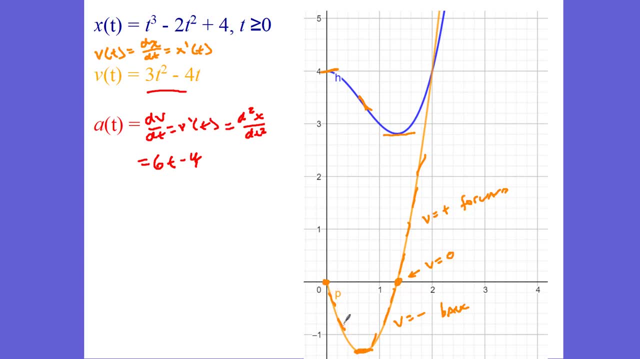 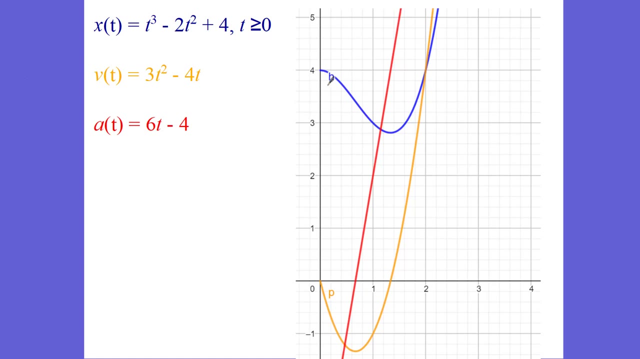 the slope of this orange graph tells you the acceleration. so you can see: the acceleration is negative, the acceleration is zero, the acceleration is positive, the acceleration is positive. okay, and so you can see when i graph that out. here are your three graphs, and how can you interpret. 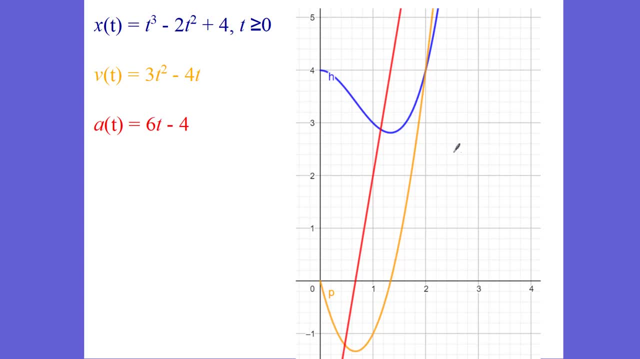 these graphs. well, i like to always look at where the slopes of the tangents are equal to zero. you can see we have a zero and a zero. that means the orange graph is at zero and zero, and then we have a zero. this graph which gives you corresponds with that zero, right there, okay, all my. 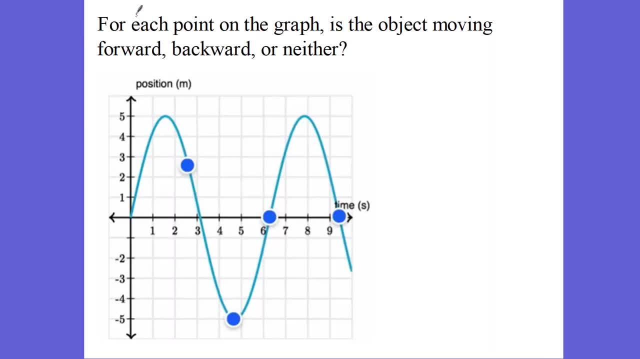 acceleration. if we take a look at at this graph, the big thing we want to do anytime we see a graph is we want to see what type of graph it is. is it a position time graph or is it a velocity time graph? because we will interpret it. 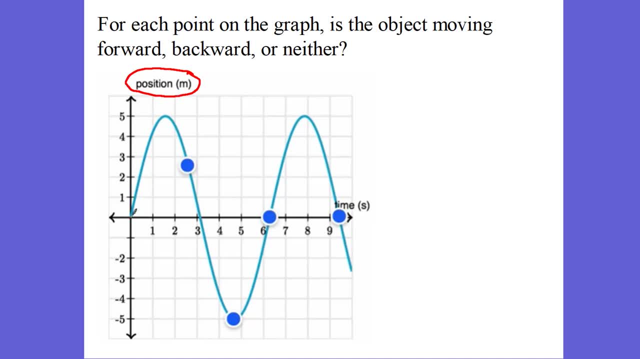 very differently. this is a position time graph. so we start out under position of zero, we're moving forward all the way to five meters, then we are moving backwards, aren't we? all the way back to position zero. then we're moving backwards, and then, right here, we're neither moving forward nor backwards, because we are. 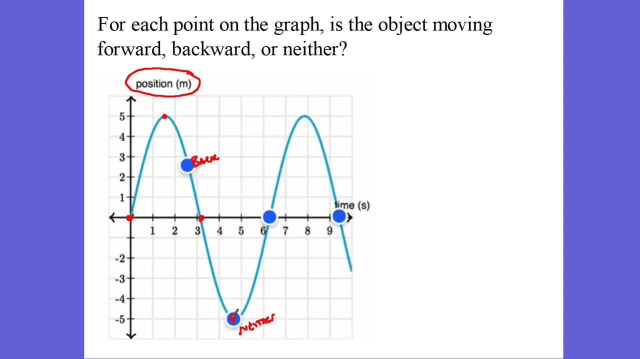 changing our direction. okay, and you can see, now we're moving backwards all the way to zero. okay, but you can see, at this instantaneous point we're moving forward and then we're moving backwards, and then we're you might say I'm not moving here. I'm not moving here, no, you're moving forward. 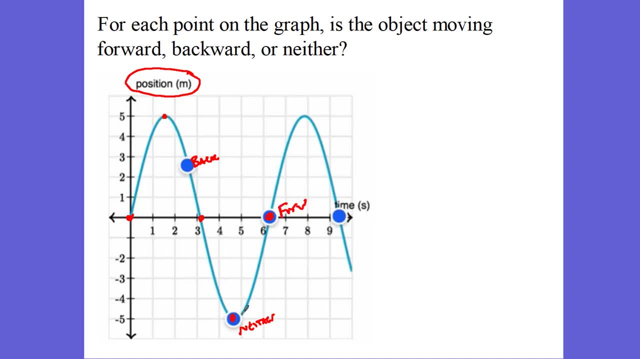 here. why are you moving forward? is you can see how we're continuing to go forward? we're going from the negative position to a positive position. we're moving forward and now, at this point in time, we're moving backwards, because we went from five meters and we're continuing to move backwards. okay, so we? 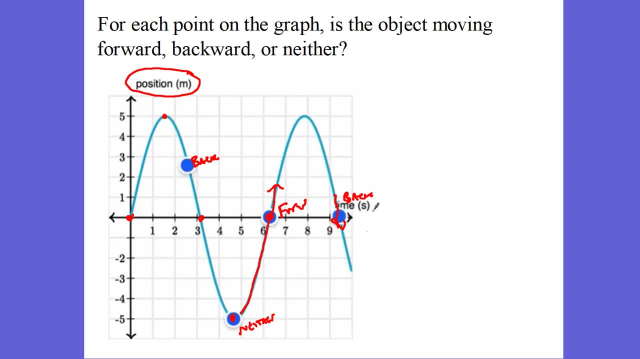 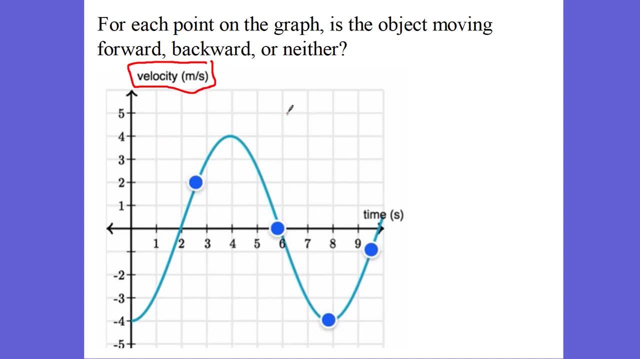 got backwards, neither forward, backward on this type of graph. you can see this graph graph. this graph is a velocity time graph, okay, and so we need to think, change your mind into talking about velocity. so we're going negative. four meters per second, okay, this is really going very fast, but in 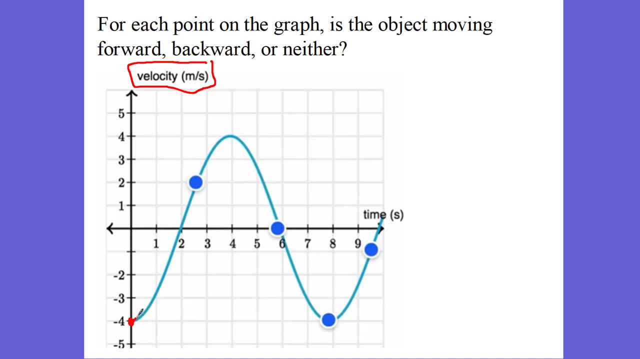 the negative direction. okay, and you can see he's slowing down all the way to zero meters per second. zero meters per second, now this we're speeding up, and now we're going positive two meters per second, which means we must be moving forward, army. now we go all the way, we're going the fastest, our speed is positive. 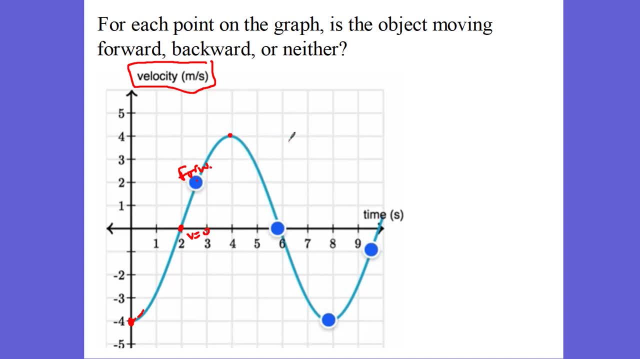 four meters per second in the positive direction, we're moving forward and we come back to a velocity of zero, and when we're going to velocity of zero we are standing still, which means we're neither going forwards nor backwards. if we're standing still at a velocity of zero, now we start moving in the negative. 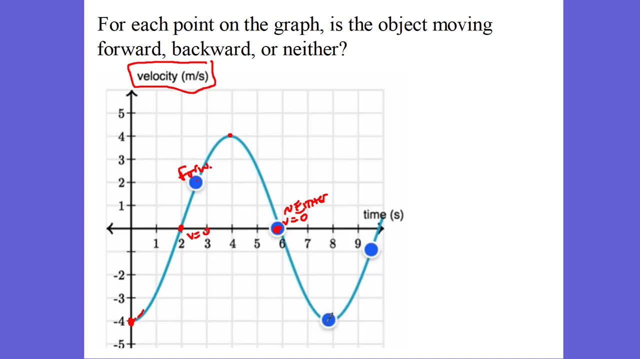 direction, because now we're moving backwards, which means, right here, we're moving backwards, we're moving negative four meters per second. we're going four meters per second in the negative direction. we're moving backwards and still, right here, we're going negative one meters per second, we're going one. 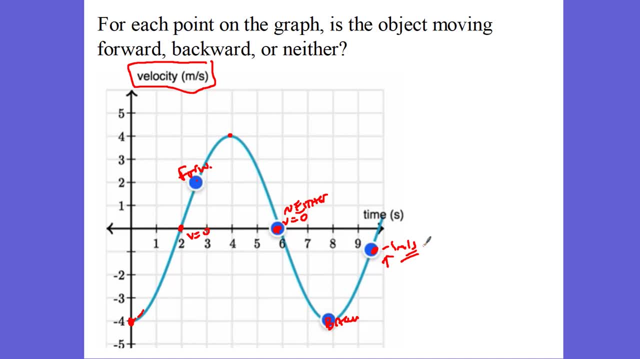 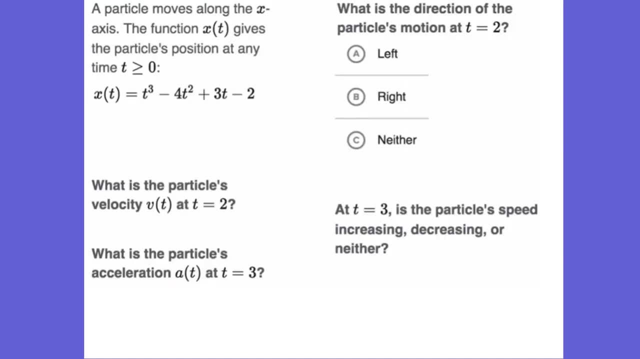 meter per second in the negative direction, which means we're still moving backwards. so we have forwards, neither backwards and backwards here. okay, I think this is one last example. here we have a particle moving in a X axis at this position function. it's a cubic function right here, and we want to. 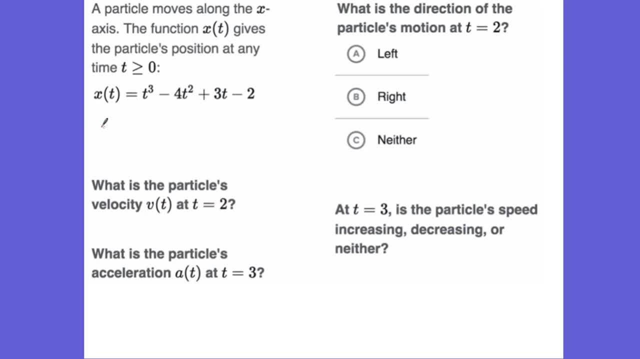 know the particles, velocity at time equals two. so how do I find the velocity with respect to time? I'm going to take the derivative of the position with respect to time, which means I have 3t squared minus 8t plus 3. I want to find. 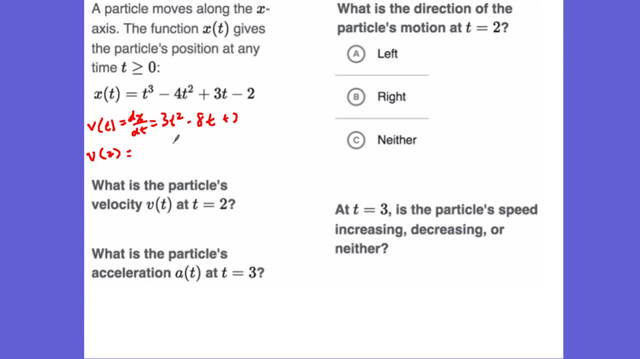 the velocity at exactly, at this instantaneous point of two, which means 3 times 2 squared minus 8 times 2 plus 3, and when I do all of this I end up getting, I believe, negative 1 meter per second. okay, you can see, 3 times 4 is 12. we have 12 minus 16 plus 3, and that's negative 1 meter per second. so the next: 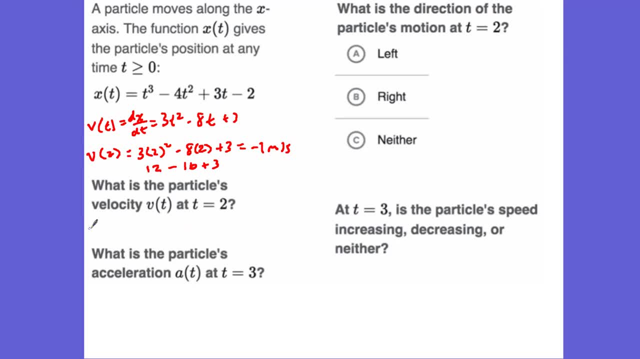 thing is, what about the acceleration? acceleration is a function of time. is the change of the velocity with respect to time the change of the velocity with respect to time? so I'm going to take this velocity function I found and take the derivative. I have 6t minus 8 and I want to know, at exactly 3 seconds of 6 times 3 minus 8. 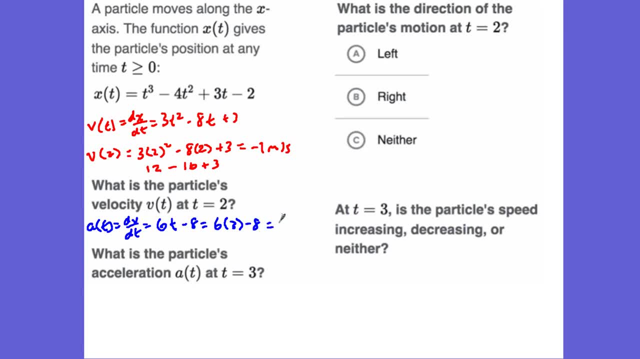 so we have 18 minus 8, which is 10 meters per second squared. okay, there's units on that. so the acceleration is positive here, that positive 3. so let's take a look at what's happening here. It says what is the direction of the particle's motion at negative 2?. 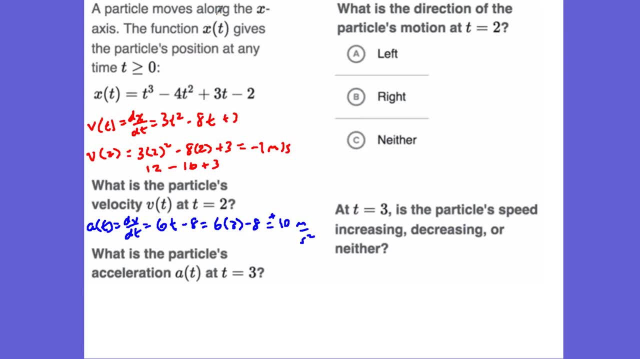 And so we said that a particle is moving along the x-axis. So you can see, right is going to be positive, left is going to be negative. We're moving negative 1 meter per second, which means we must be moving to the left. 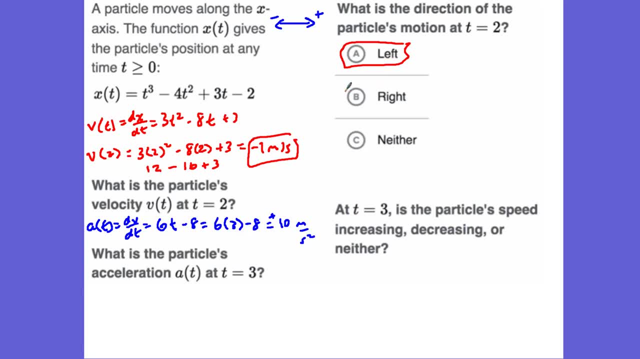 We must be moving to the left for this answer here. And then, what do I know about the particle's speed? The particle's speed, it's positive 10 meters per second squared, which means the velocity is changing in a positive way. The velocity is changing in a positive way. 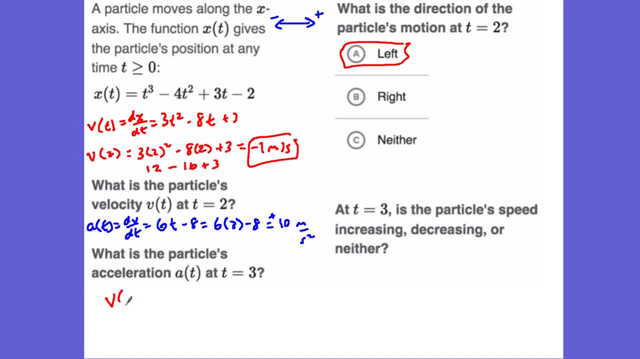 Now I want to check out the velocity at this: 3 seconds, And so I have 3 times 3 squared minus 8 times 3 plus 3.. I can go back to this velocity function right here, So I have 3.. 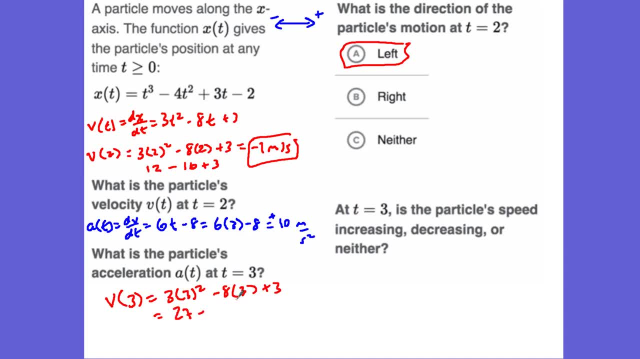 8 times 9,, that's 27,, minus 8 times 3, that is 24, plus 3.. And so you can see how, here I'm positive: 6 meters per second. So the velocity is positive. The acceleration is positive, which means the speed must be increasing here. 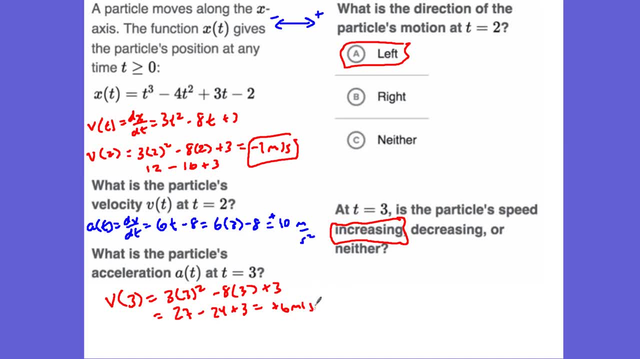 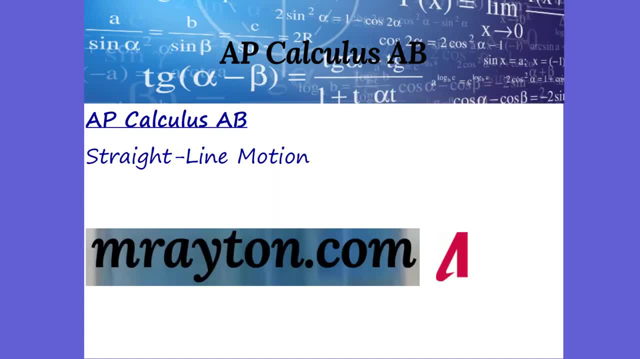 because those are both matching that positive and that positive. So this is a lot of physics in the straight line motion. It's not that hard. We're just taking derivatives. Going from position to velocity to acceleration is derivative, derivative derivative. 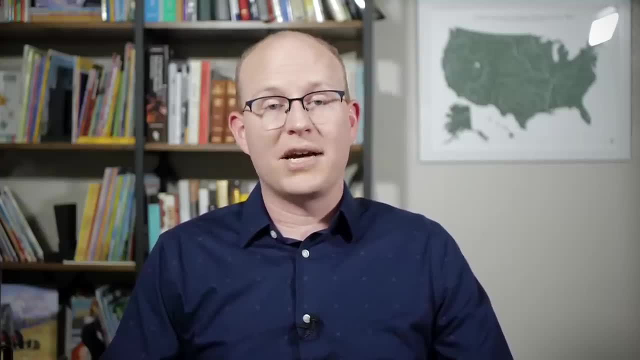 All pipes carrying fluids experience losses of pressure caused by friction and turbulence of the flow. It affects seemingly simple things like the plumbing in your house all the way up to the design of massive, way more complex long-distance pipelines. I've talked about many of the challenges. 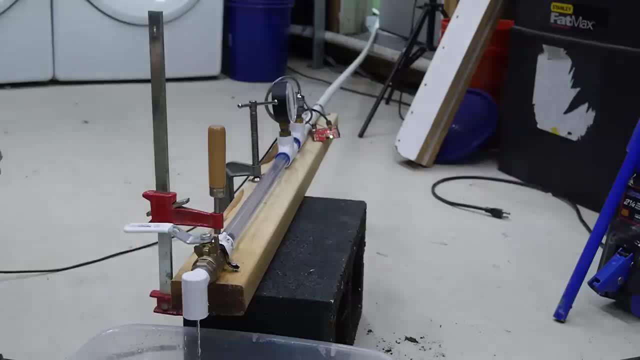 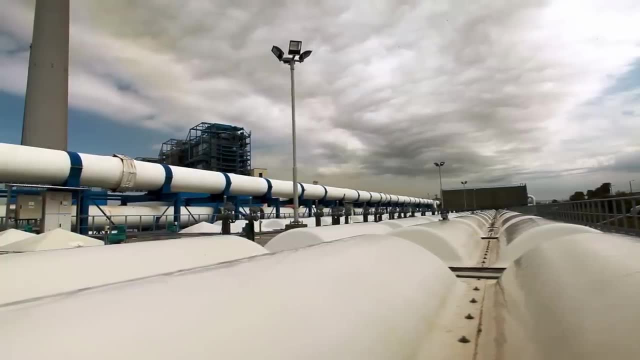 engineers face in designing pipe systems, including water hammer, air entrainment and thrust forces- but I've never talked about the factors affecting how much fluid actually flows through a pipe and the pressures at which that occurs. So today we're going to have a little fun. 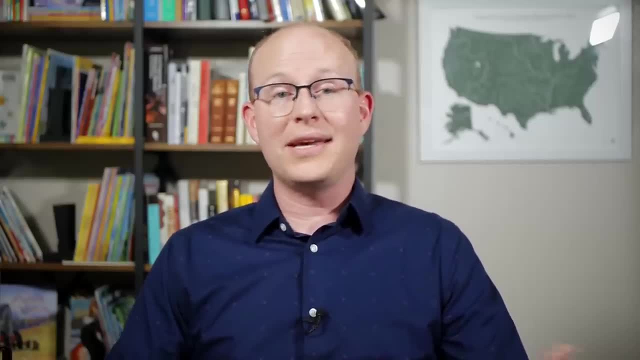 test out some different configurations of piping and see how well the engineering equations can predict the pressure and flow. Even if you're not going to use the equations, hopefully you'll gain some intuition from seeing how they work in a real situation. I'm Grady and this is Practical Engineering In today's episode. 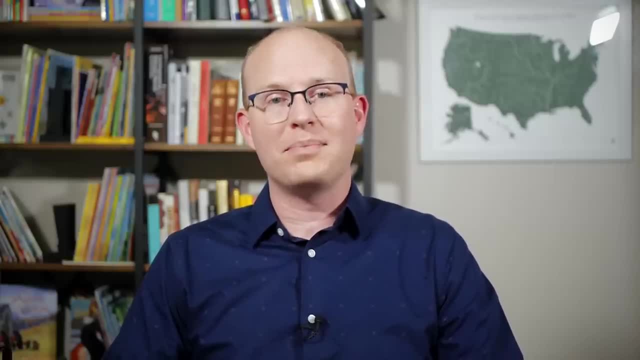 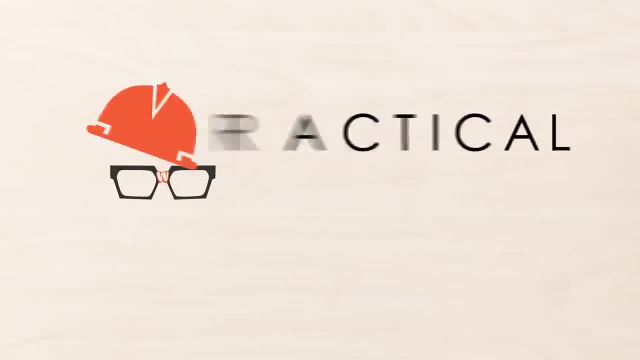 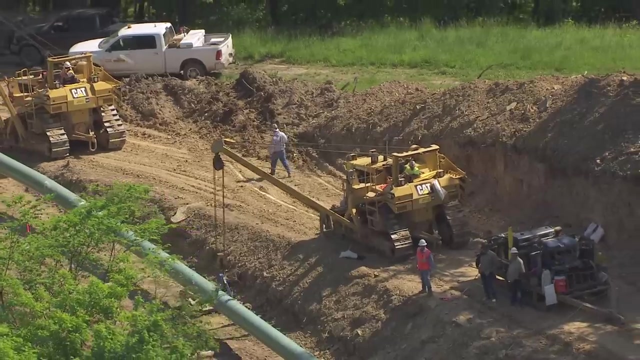 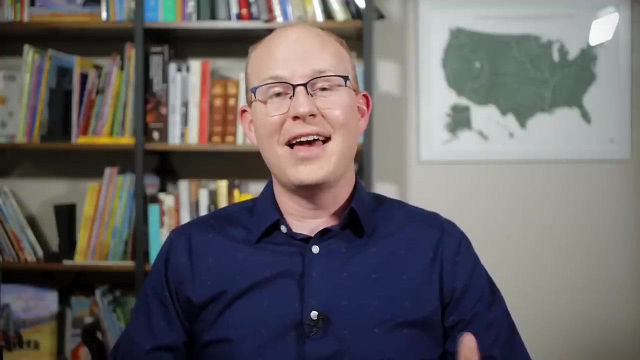 we're talking about closed conduit hydraulics and pressure drop in pipes. This video is sponsored by HelloFresh, America's number one meal kit. More on that later. I love engineering analogies and in this case there are lots of similarities between. 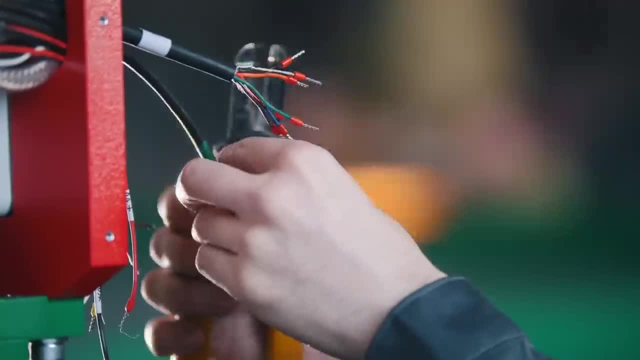 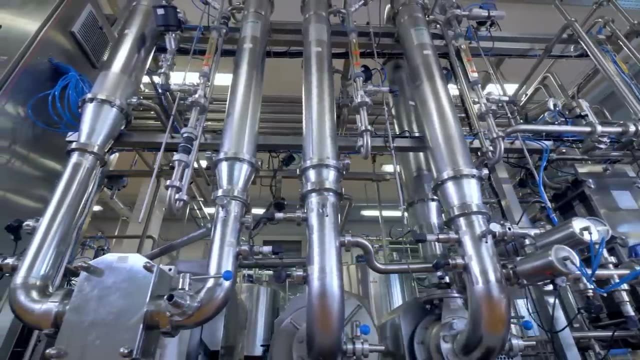 electrical circuits and fluids in pipes, Just like all conventional conductors, have some resistance to the flow of current. all pipes impart some resistance to the flow of fluid inside, usually in the flow of the pipe. So if you're not familiar with the flow of current, you'll know that the